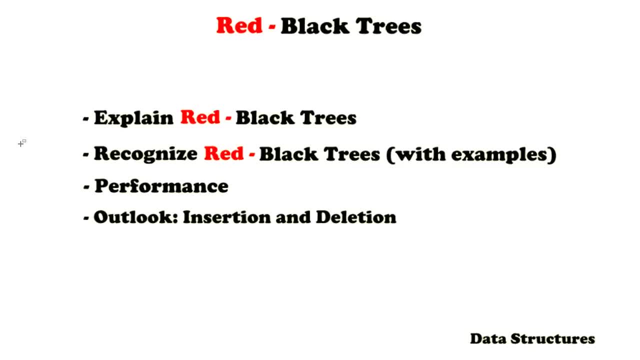 Hi there, my name is Mr Coat, and in this video we're going to talk about red-black trees, and before going into the details, let me first give you an overview of what I'm going to talk about. So first of all, of course, I'm going to explain what red-black trees are, Then we're going to 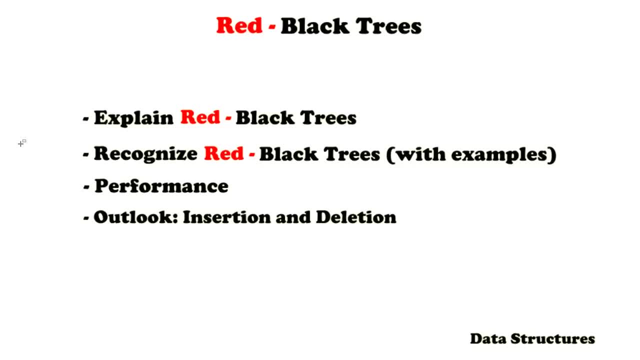 recognize red-black trees and, based on a few examples and based on this section, you will actually master to recognize what properties a red-black tree should actually satisfy. Then we're going to have a talk about the performance and finally we're going to have a little outlook. 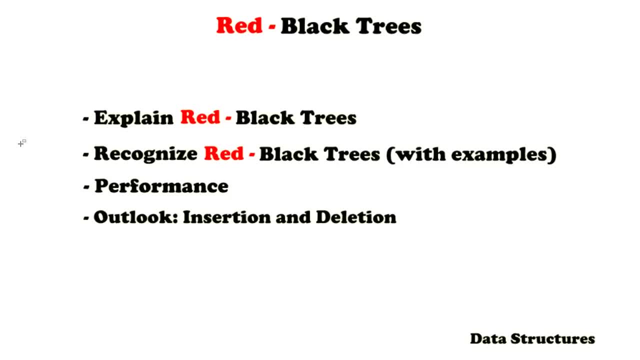 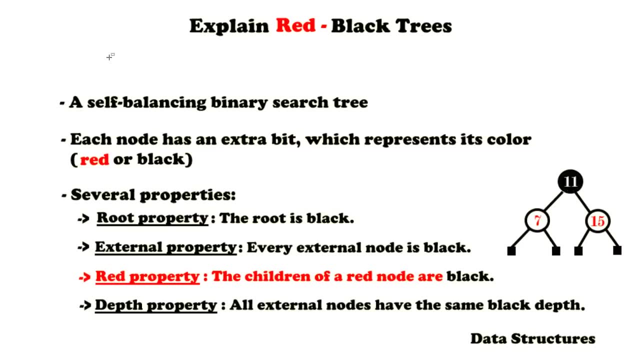 on both insertion and deletion, and we'll come to that. But first let's explain what red-black trees are. So a red-black tree is a self-balancing binary search. Each tree and each node has an extra bit. and this is special for a red-black tree because 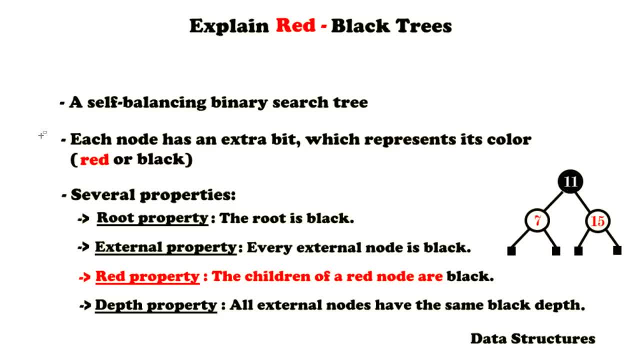 this extra bit represents its color. It's either red or black, and that's why they're called red-black trees, of course, And each red-black tree should satisfy several properties. There are four of them, and the first one is the root property, which says that the root 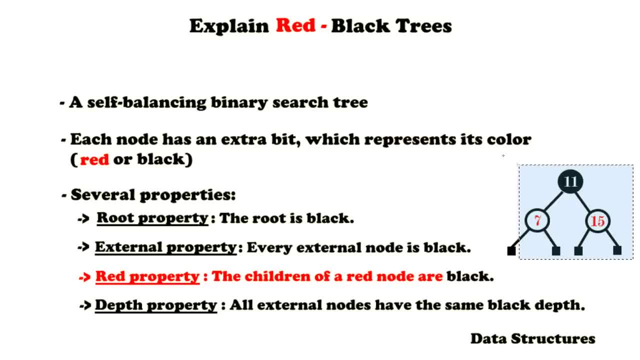 is black. So on the right here I have a small example. Here you see that the root node is actually black. Then there is the external property, which says that every external node is black, and I indicated that by these black squares at the bottom. These are the external. 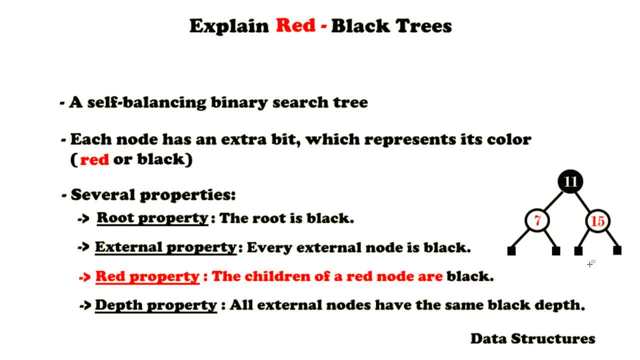 nodes and they represent the black external nodes. So this property is black. This property should always hold as well. Then there is the red property, which says that the children of a red node are always black. So for this red node, its children are of course black because these are the external nodes and I made them black. But in general, 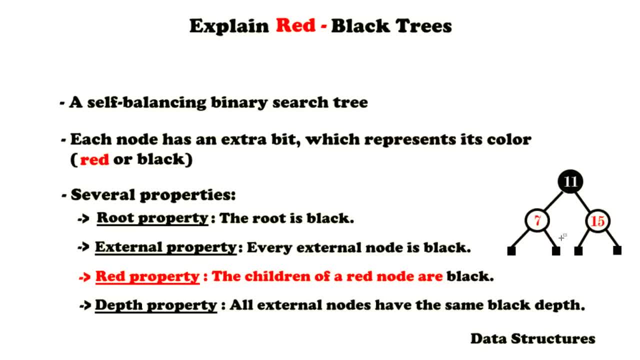 it must hold that within any tree, if there is a red node, the children of a red node are black, Then the children of it should be black. And then, finally, we have the depth property, which says that all external nodes have the same black depth, And by this I mean that the number of proper ancestors that are black 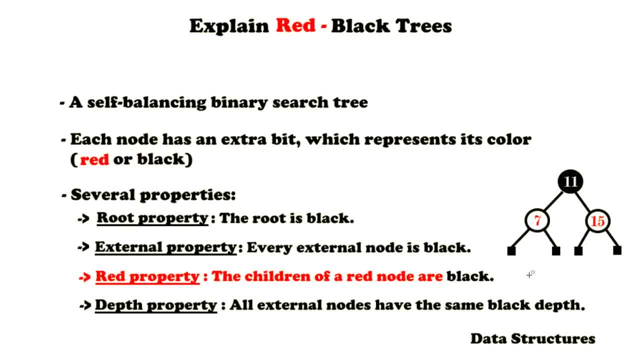 represents the black depth. So, for example, in this red-black tree the black depth is one, Because the external nodes don't count. and for every path to an external node in this red-black tree, there is only the root node that counts as a black node. So for every 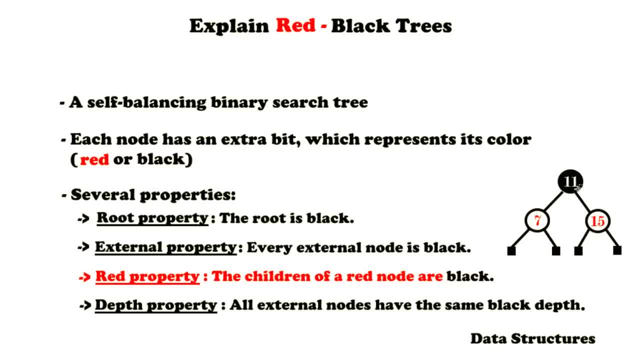 path there is no other black node except for the external node. So for every path the black depth will be one. So that's the black depth for the red-black tree. And because this red-black tree is black, because every external node has the same black depth, this property holds. 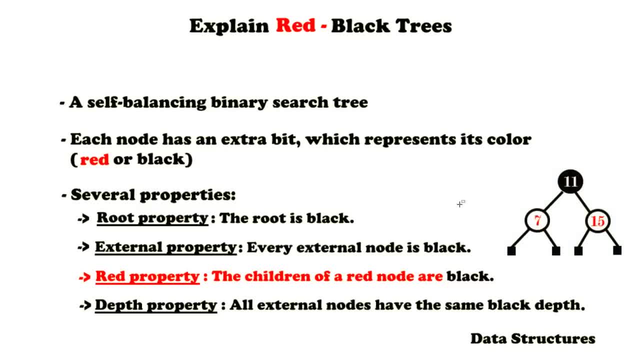 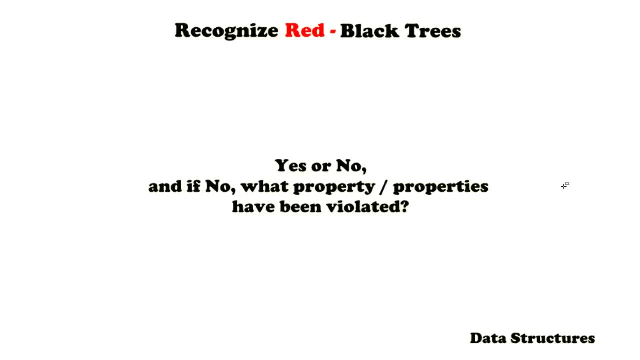 So for this little example, all the properties hold, and for every red-black tree these properties should hold. Okay, so let's now move on to the next section, and for this I've prepared a few examples, and these examples can either be a red-black tree or they're not. 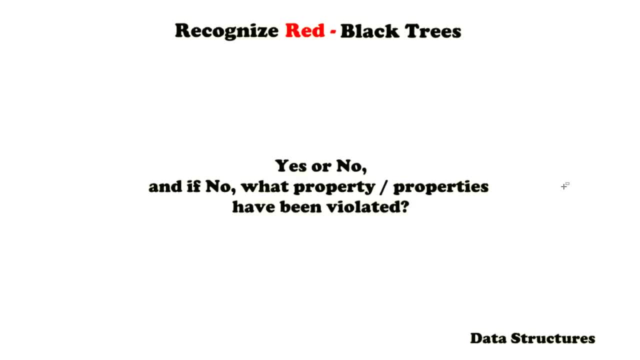 Because some property or some properties have been violated. So, for every example- and these are four examples- we're going to answer the following question: so, either yes or no, is it a red-black tree? and, if not, please also indicate what property or what properties have been violated. 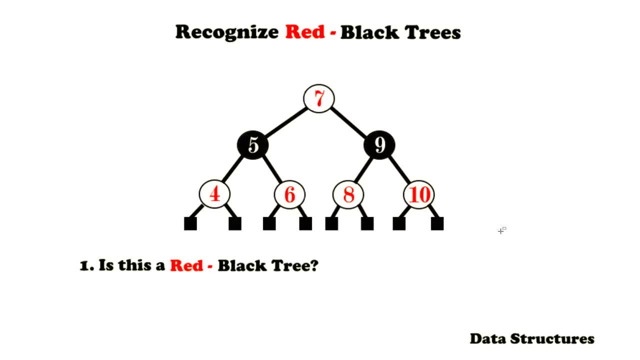 So let's move on to the first example. This is the first red-black tree. So for you, the question: is: this a red-black tree? And if you want to think about this, please pause the video and do think about it. Write down your answer or just keep it in mind and press play again if you. 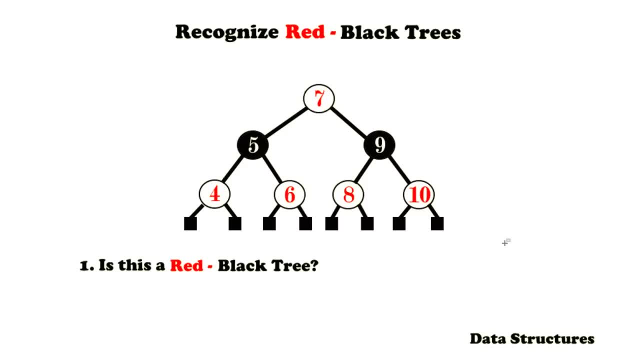 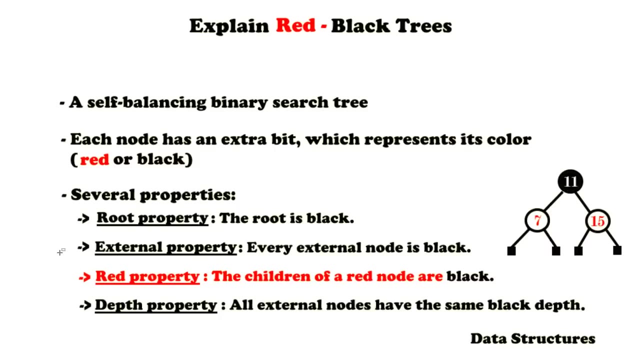 want to see the answer, because that's what I'm going to continue with now. So the answer is no. This is not a red-black tree because the root property has been violated. If we have a look again at the list of properties that a red-black tree should satisfy, 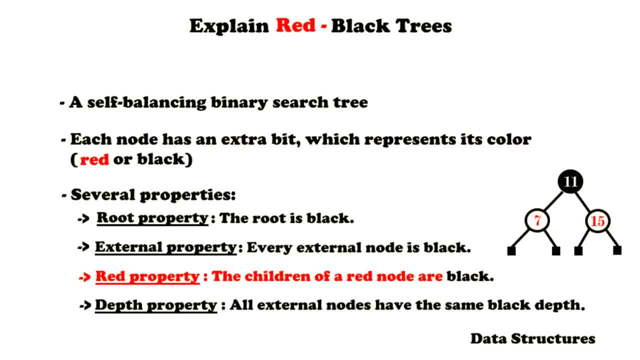 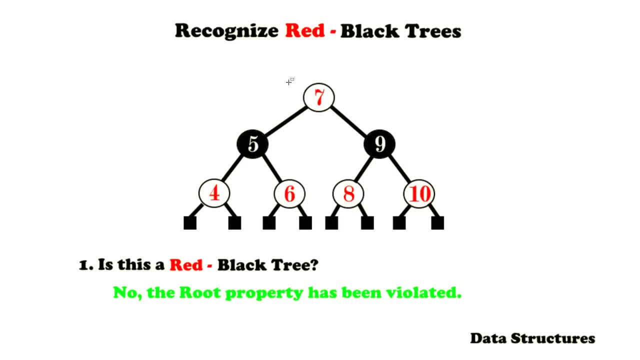 The root property implies that the root of a red-black tree should be black, And clearly this root node is not black. So the root property has been violated and thus this is not a red-black tree. So the more the black depth holds, also the red property holds and every external node 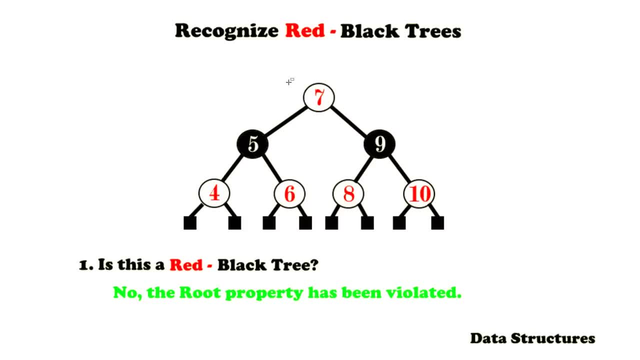 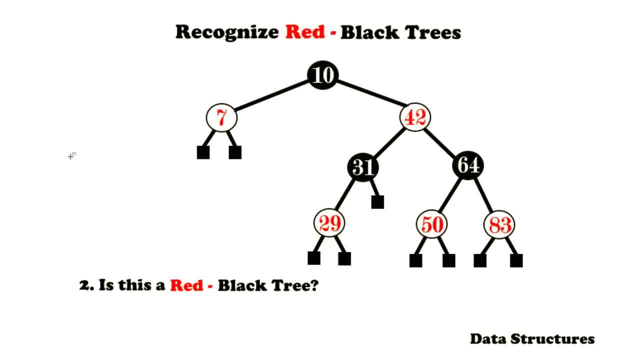 is black, So the external property also holds. Okay, so let's move on to the second example. And now the question again: is this a red-black tree? Again, if you want to think about this past the video, come back If you know the answer. and for now I will continue with what the answer to this question? 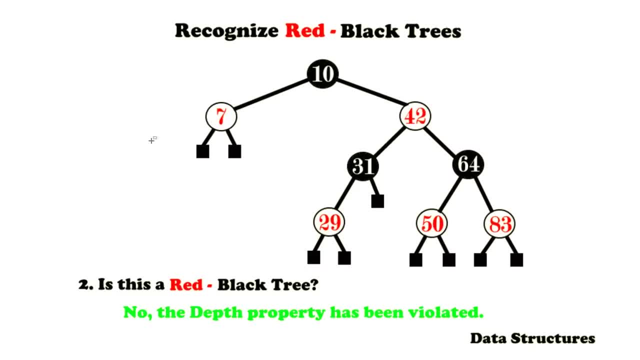 is. So the answer is again no. The depth property has been violated. so it's not a red-black tree. And this is the case because, well, if we go along every path to an external node and we count the amount of proper black entities, 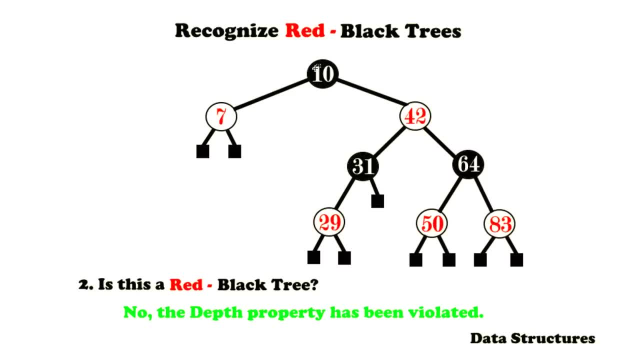 Ancestors. We don't always get the same answer. Let's, for example, go along this path: So the root node is black, So we're going to count 1.. Then at this point, the external nodes don't count. So for 7, the black depth is 1.. 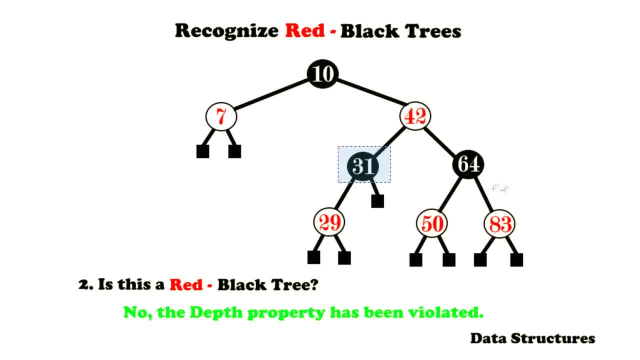 And if we go along this path, We encounter two more nodes- Black nodes along each of these paths. So the total number of black nodes that we find will be 2 here, 2 here and 2 here. And because there is a difference, this binary search tree must be unbalanced. 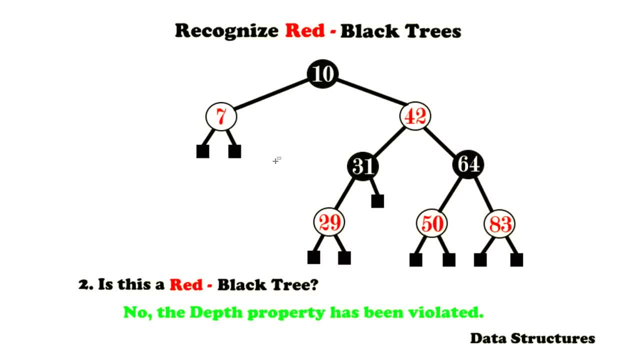 So depth property has been violated and therefore this is not a red-black tree. So that's the answer. Let's move on to the third one. So I didn't change a lot compared to the previous one. Just look at it: This is the previous one and this is the third example. 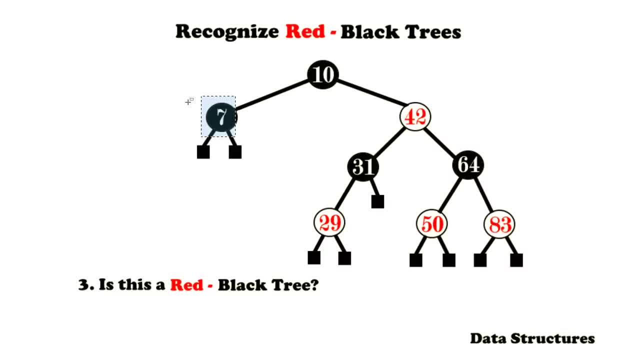 The only thing I changed is this node. I recolored it. It was red and now it's black. So in the previous example The answer was no to the question because the depth property didn't fault. But is this a red-black tree? 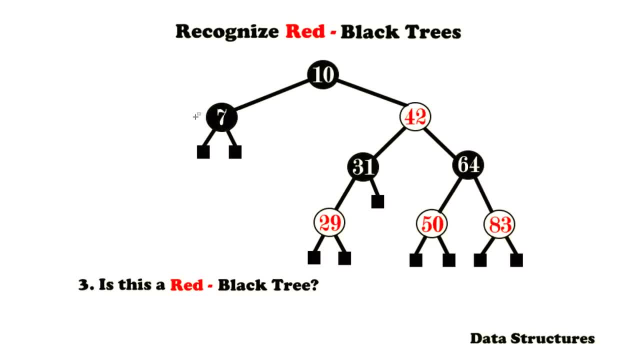 And it sounds like I'm going to sound like Dora the Explorer with all these binary questions, But these are, of course, important questions in order to master to recognize what red-black trees are and what aren't red-black trees. So the answer to this question is yes, this is a red-black tree. because? well, now the because. 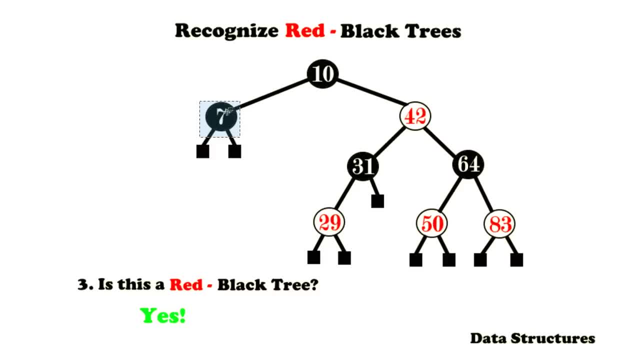 this path also has a black depth of 2,. for every path the black depth will be 2.. So the depth property has been satisfied and also the root node is black and the external nodes are black. And the root nodes are black And the external nodes are black. 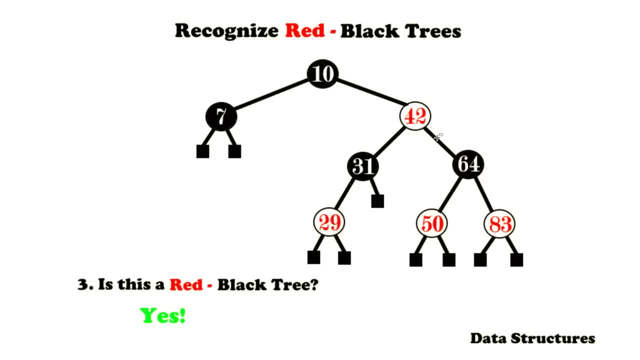 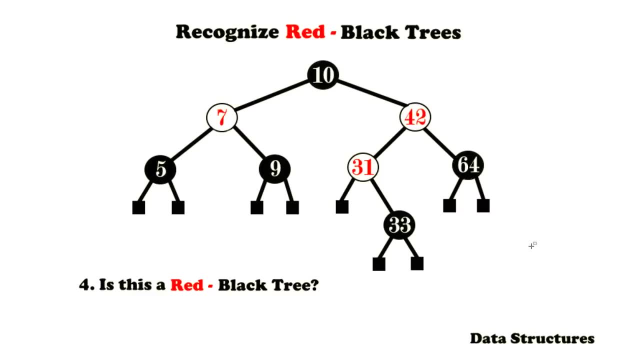 And the root, the red property, has been satisfied as well. So okay, let's now move on to the last example. The question for you is now again: yes, I'm Dora the Explorer. Is this a red-black tree Press, pause again and play when you're done. 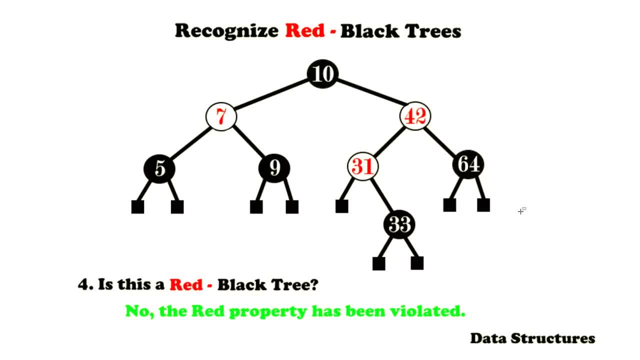 But the answer to this question is no, Because the red property has been violated. Well, let's just have a look at this. This red node has, so wait again for the red property. it must hold that the children of a red node are black. 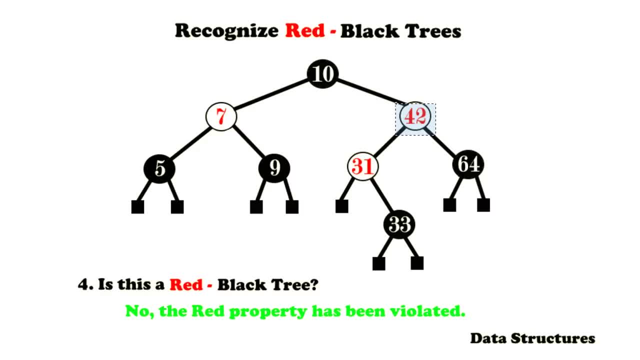 And for this node its children are black. For this node it doesn't hold that its children are black, Because 31 is a child, 31 is a child And it's red. And furthermore, for 31 its children are black, But because for this one it doesn't hold that all its children are black. the red property: 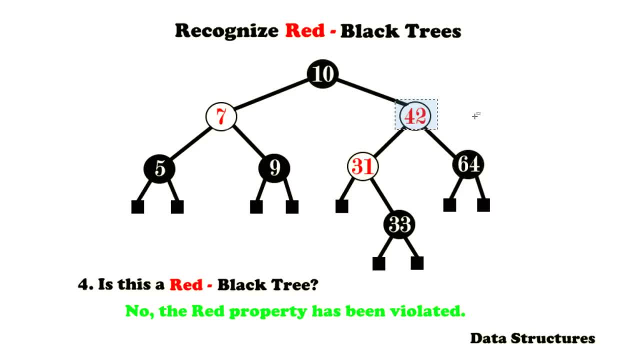 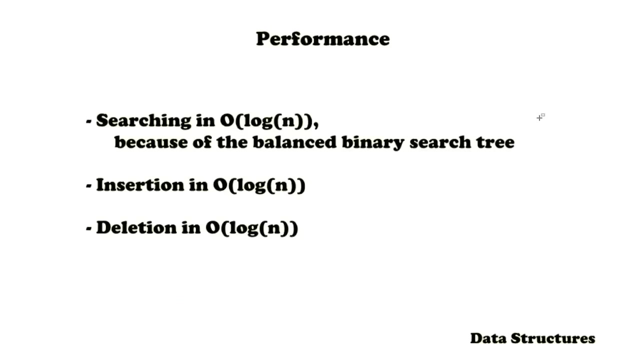 has been violated, So this is not a red-black tree. So now that we have had four examples, I think that you've mastered how to recognize red-black trees, Or whether they aren't, based on these four properties. So let's move on now to the performance of red-black trees. 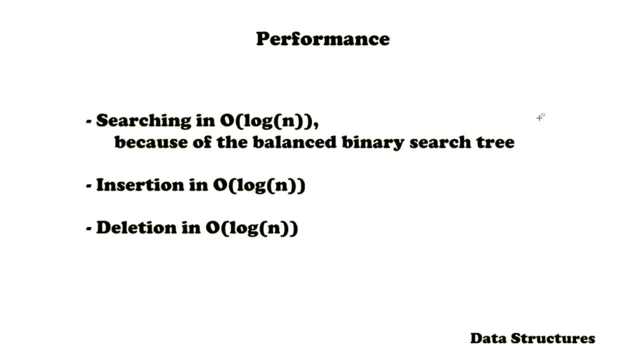 And searching in red-black trees can be performed in O log n, In which n is the amount of nodes in the red-black tree, And this is because of the balanced binary search tree. A red-black tree is essentially a binary search tree. A red-black tree is essentially a binary search tree. 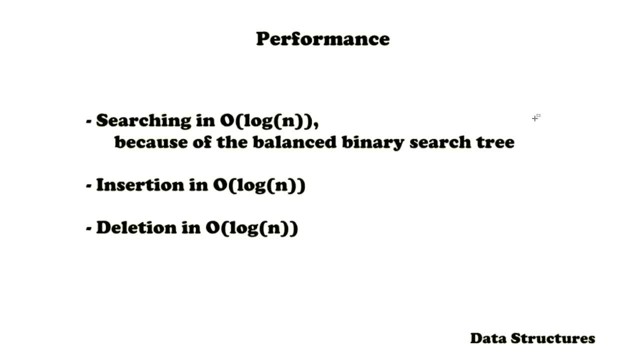 A red-black tree is essentially a self-balancing binary search tree. So whenever you go along a path searching for a specific node, you have to make a decision. Are you going to the left half of the tree or the right half? And if you make this decision, so if it's smaller, if the number is smaller than the? 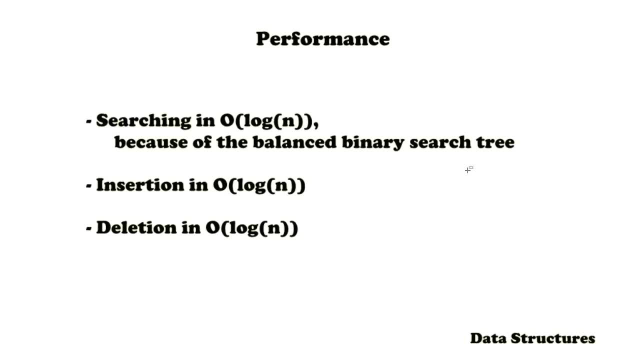 current node you're at, then you're throwing half of the nodes away each time. So, moving along this amount of nodes and going through the path, you throw half of the nodes away And therefore the amount is reduced. logarithmic And therefore searching is done in O log n. 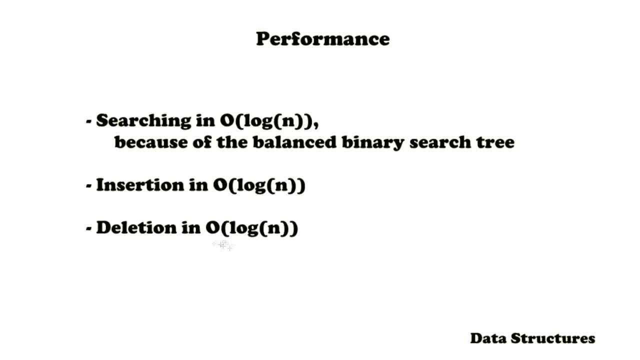 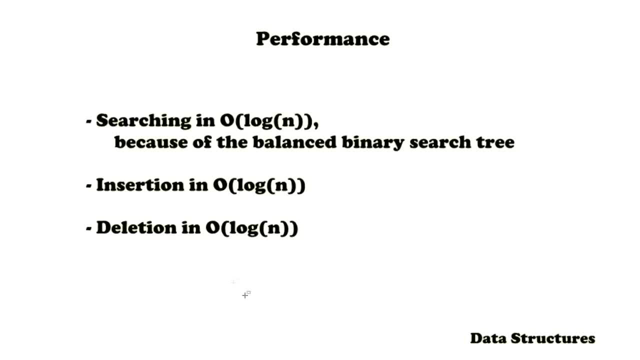 And then insertion and deletion are also done in O log n, But insertion and deletion are two operations we didn't talk about yet, And about that that's going to be something for the outlook, Because I didn't include these subjects yet into this video, because I thought this would